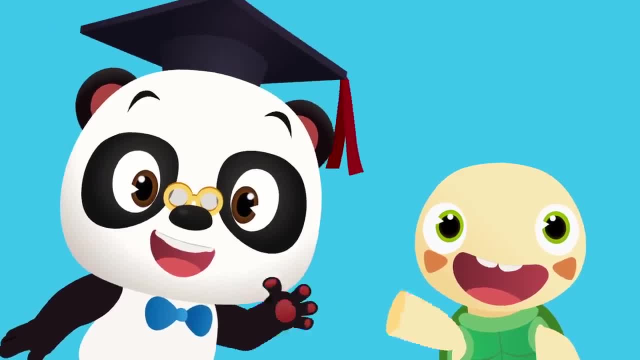 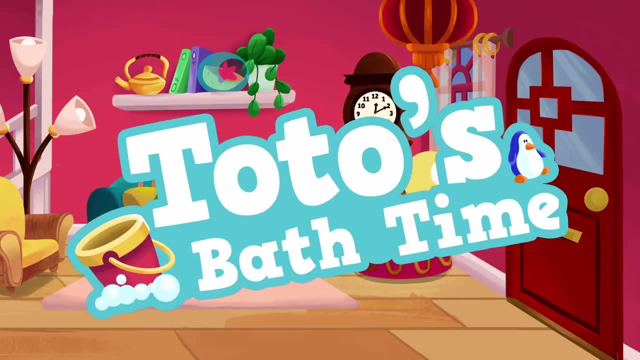 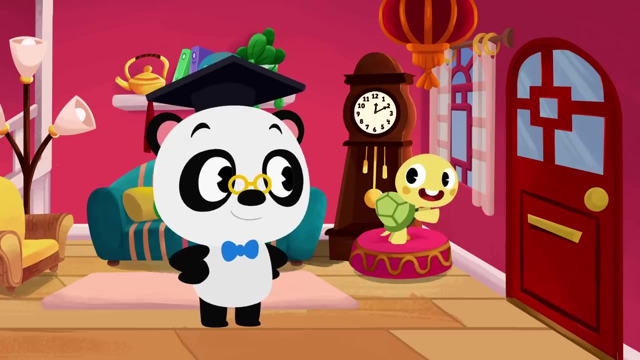 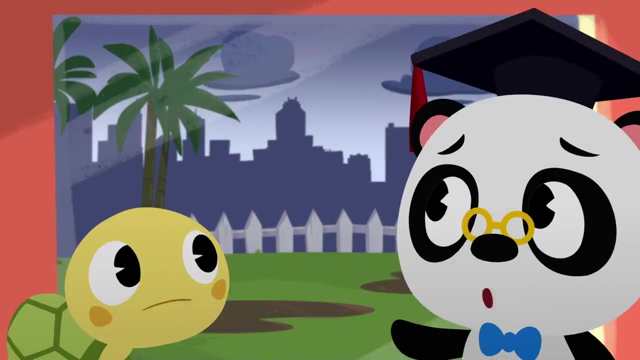 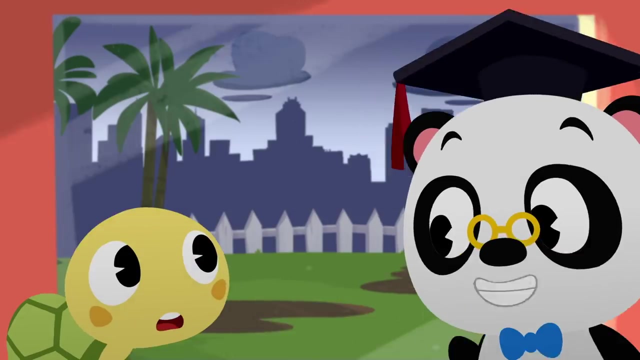 Search for Dr Panda. Yay Morning, Toto Playtime Outside, Outside- Aww, what a shame We can't play outside in this weather, Toto. Aww, no playtime. No worries, Toto, There's lots of fun things to do inside the house. 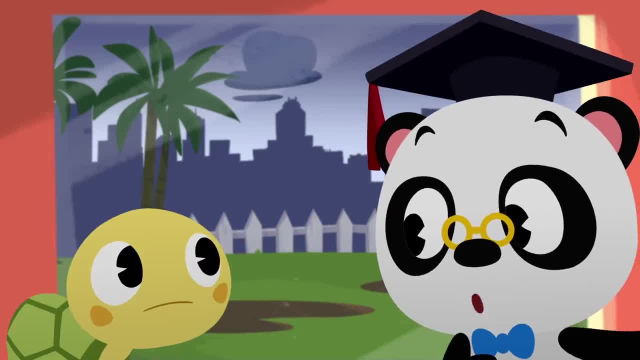 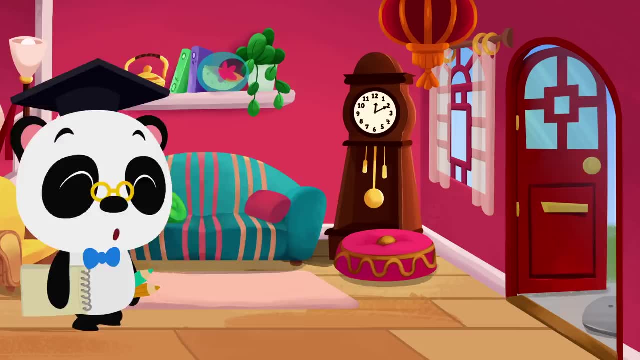 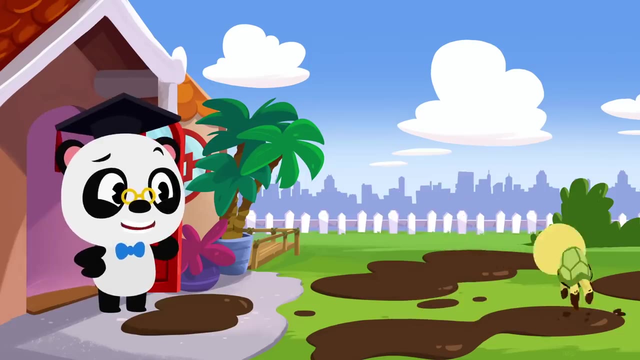 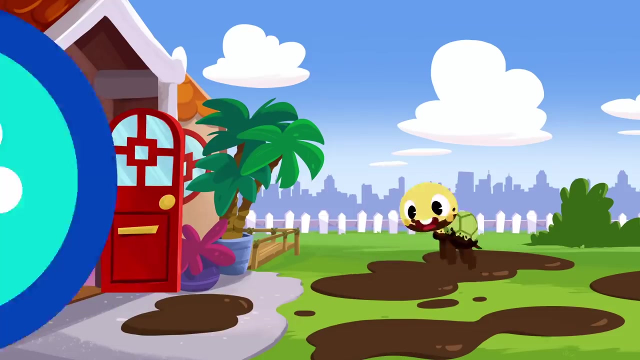 How about some drawing? I'll go and get some paper and pens. Here we go. What shall we draw first? Toto, I guess it stopped raining. Have fun playing in the mud, Toto. Hmm, I wonder if Toto's still playing in the mud. 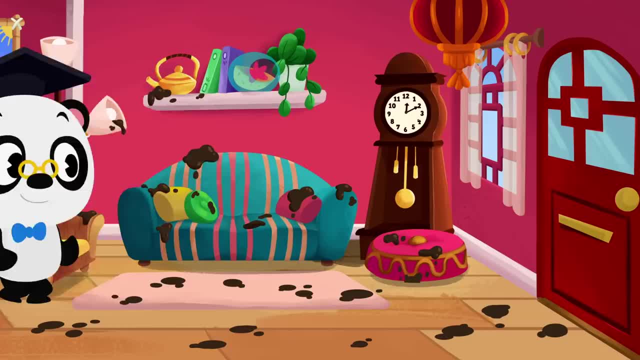 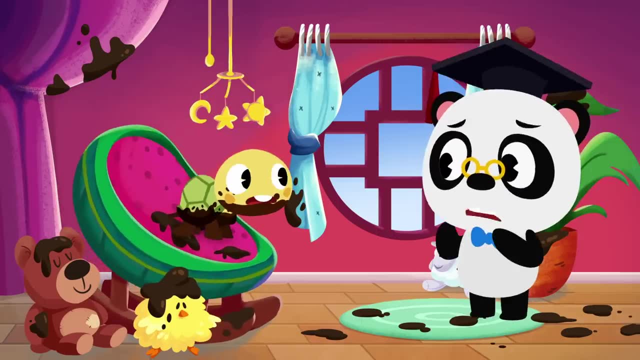 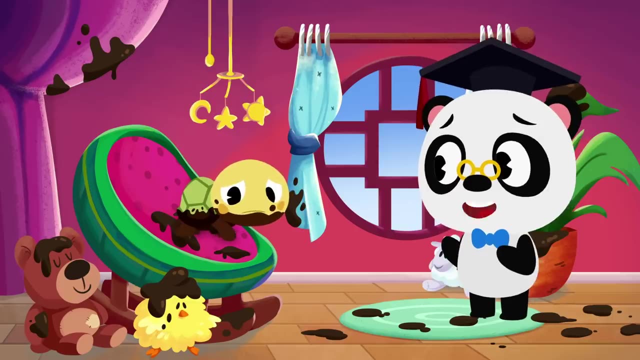 I sure don't want him to walk into the house with his feet alldirty. Toto, What are you doing? You're making everything dirty. Oops, Sorry, Aw, no worries, We can clean it up, But first we have to get you clean. 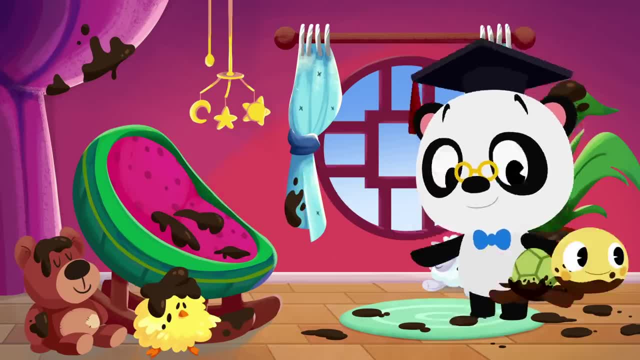 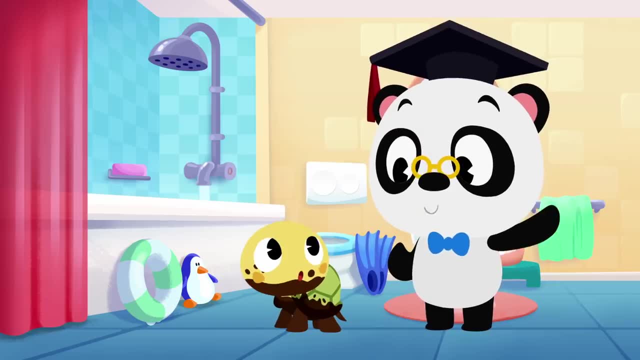 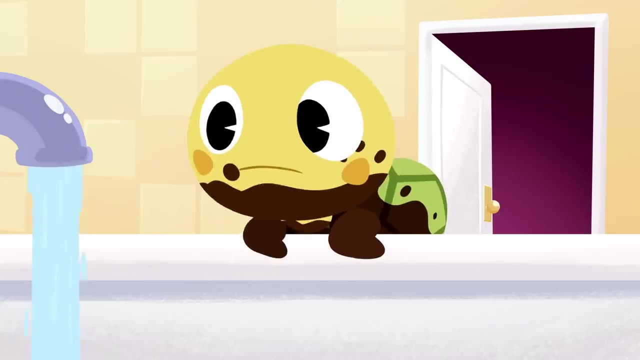 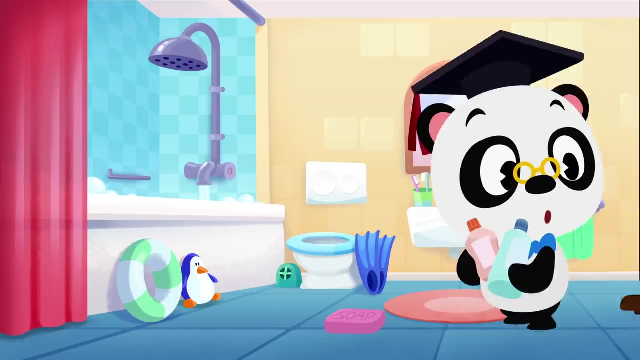 Time for a bath. You'll have to wait a bit for the bath to fill up. Toto, I'll go get some bubble bath to make some bubbles. Huh, Toto, Where are you going? Toto, Come back. 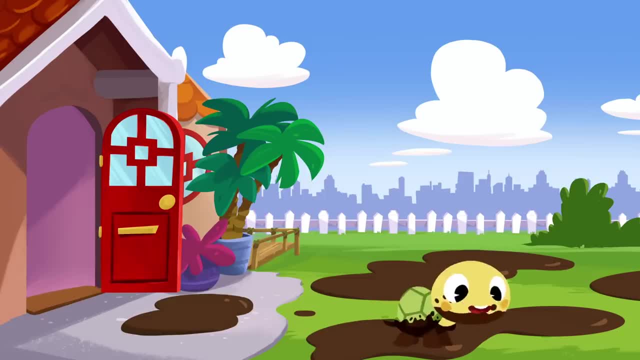 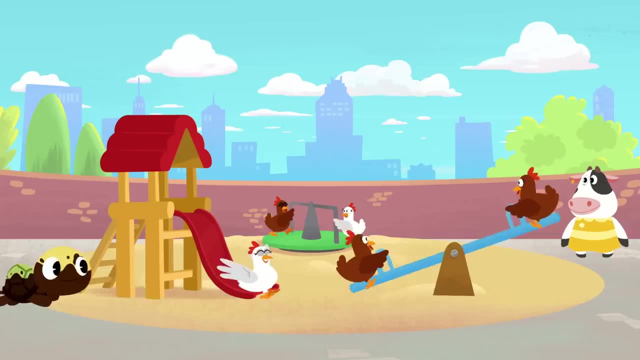 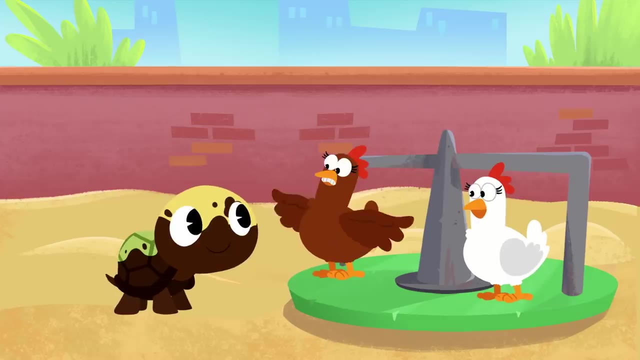 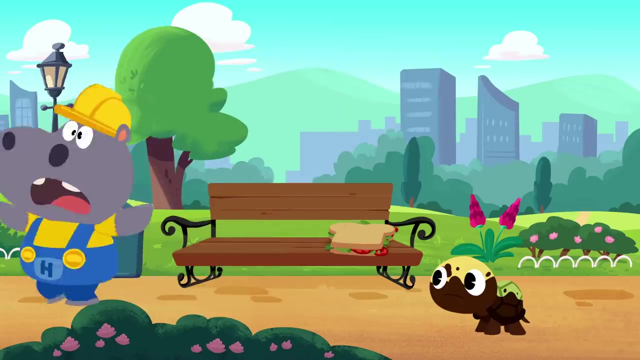 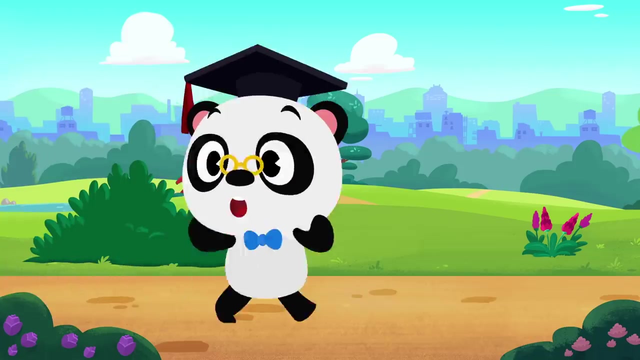 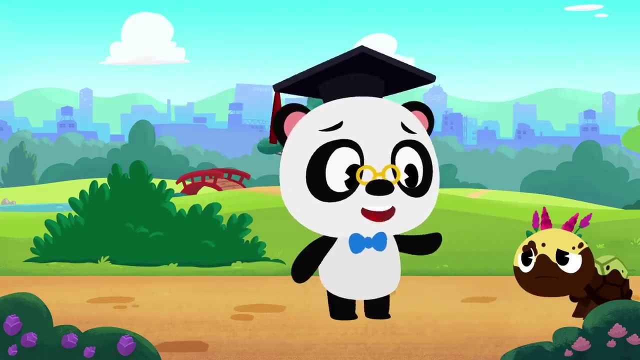 Playtime Outside Chickens. Playtime Chickens. Aww, no playtime, Hoopa, Playtime, No playtime Toto Toto, Hey Hoopa, Have you seen To To There you are. 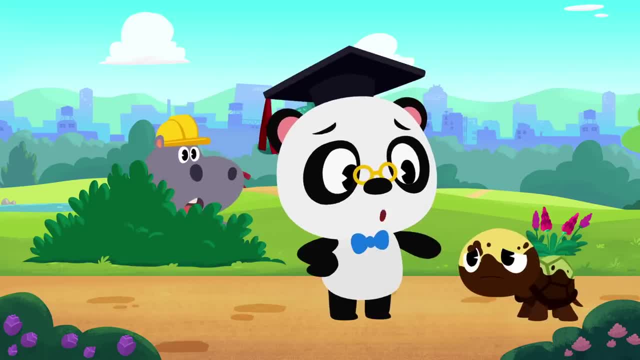 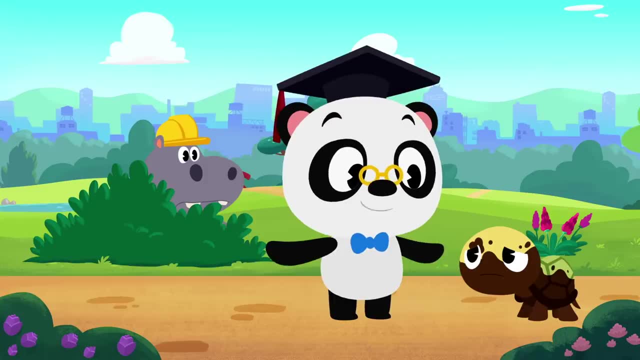 You're so covered in mud I didn't see you. No playtime. Aww, I get it. No one wants to play with you because you're so muddy And Hoopa didn't even recognize you. I bet you're ready for your bath now, aren't ya? 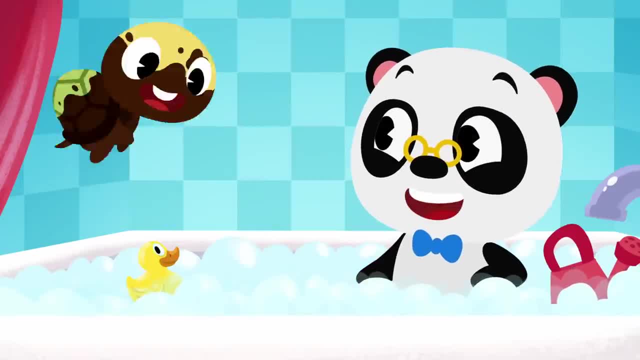 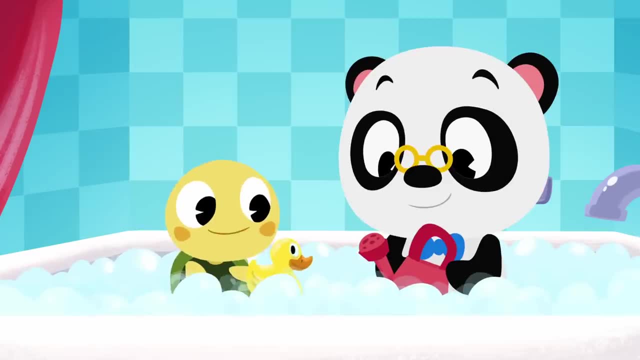 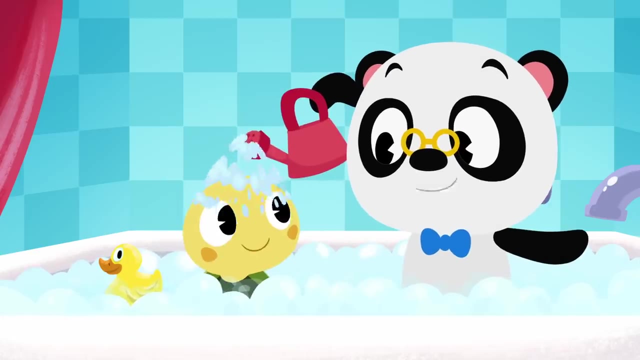 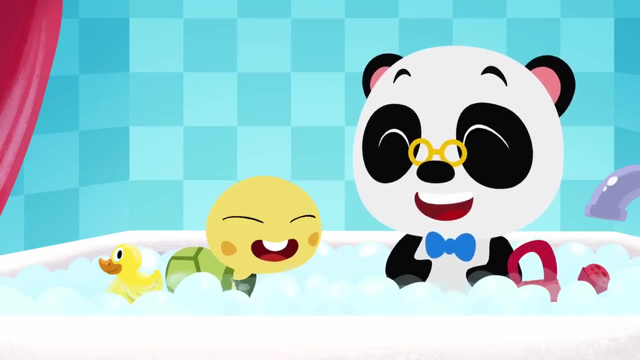 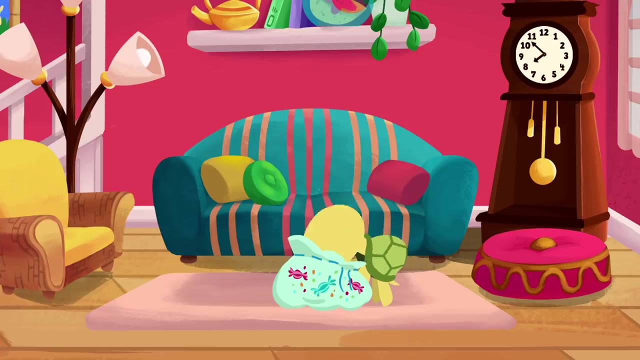 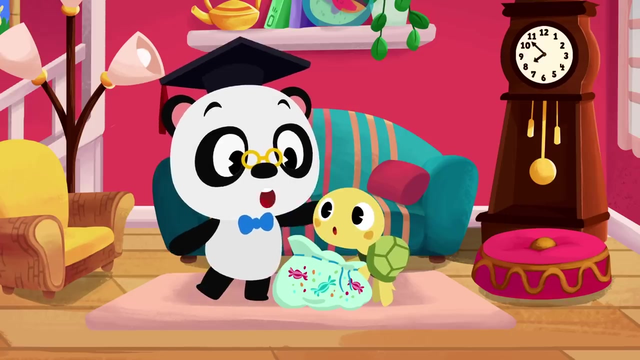 Toto Whee Playtime. Baa Baa Bubbles. See, Toto, Playing inside can be nice, Can be just as much fun as playing outside. Yeah, Yum Candy, No more candy. Never mind Toto, It's bedtime anyway. 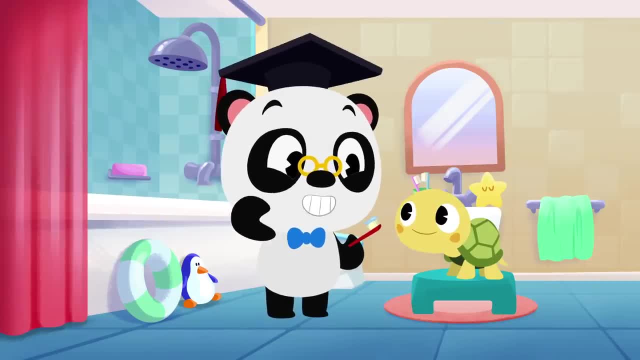 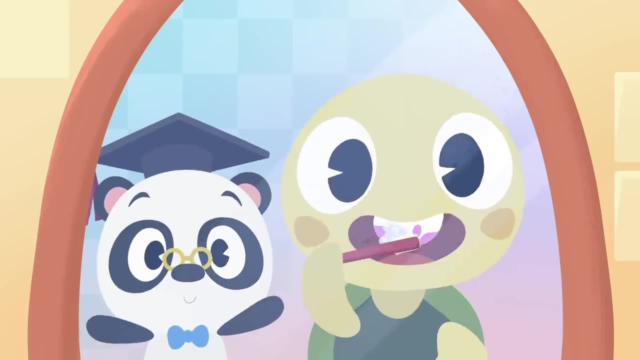 Alright, Toto, Let's see those teeth. Awww, Uh-oh, Look at all that sticky candy. Good thing we brush our teeth before we go to bed, Ready for the tooth brushing rhyme Up, down and all around. 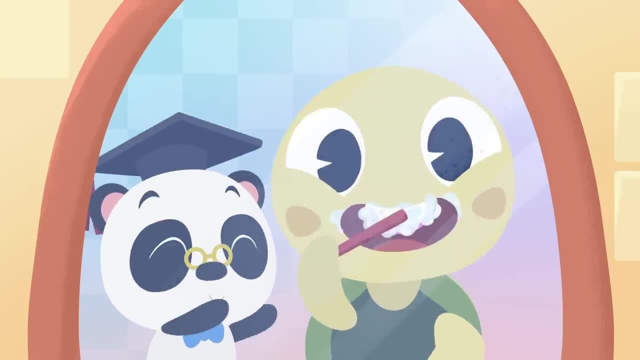 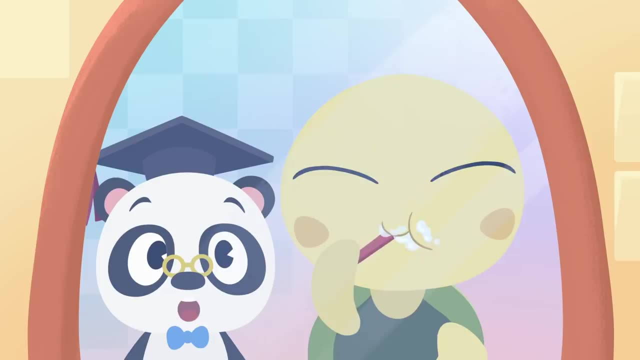 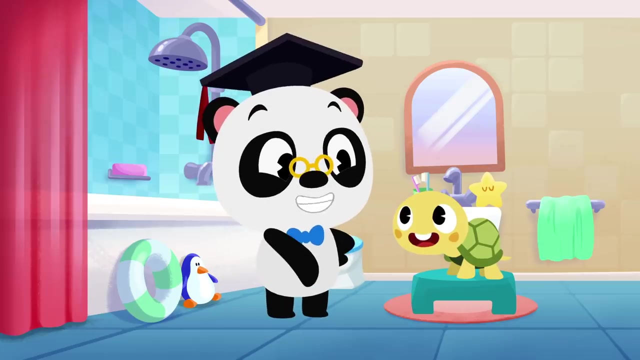 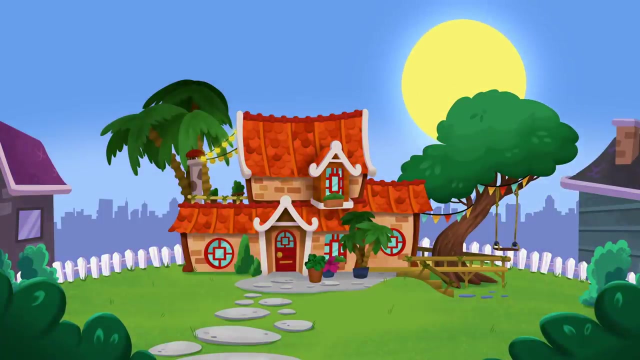 Up down and all around, Up down and all around. One last time, Up down and all around. Now rinse- Awesome, Your teeth are sparkling clean again, Toto. Yay, Good morning Toto. 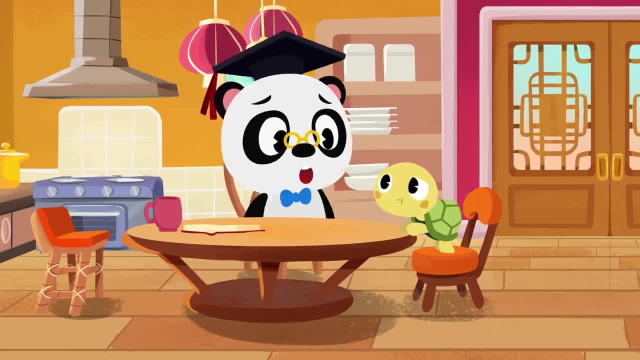 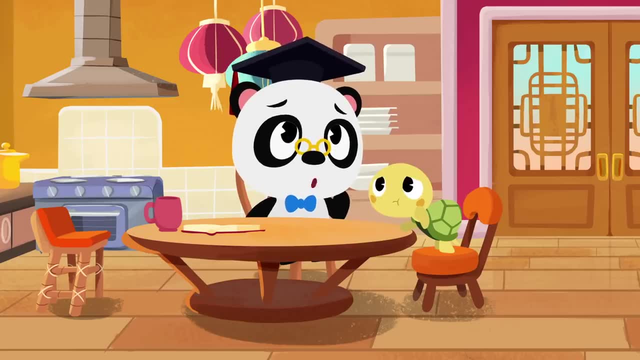 Uh Oh, what's wrong, Toto. Uh Oh, your tooth hurts. Hmm, maybe you ate too much candy. Too much candy is bad for your teeth. No worries, Toto, I know who can help The dentist. 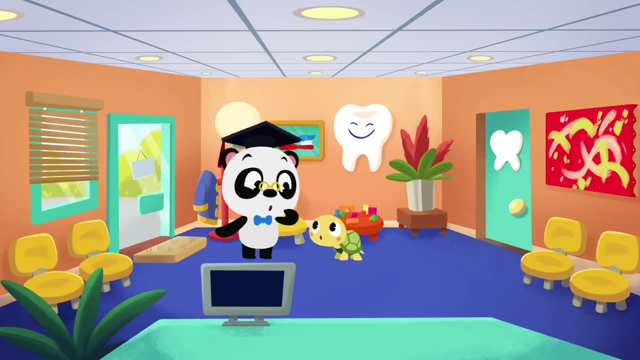 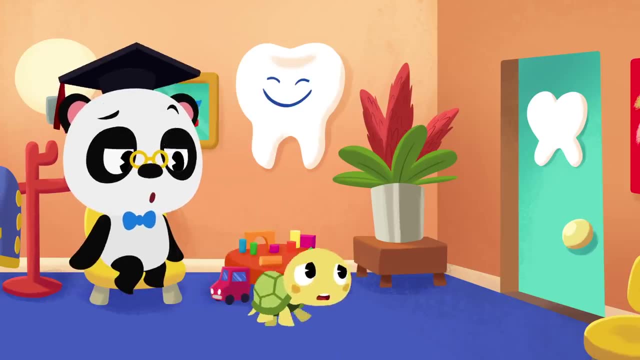 The dentist is a special doctor for your teeth. He can take the pain away and tell us what's wrong with your teeth. Those noises are just the dentist's tools, Toto, They make all kinds of funny noises, Nothing to be worried about. 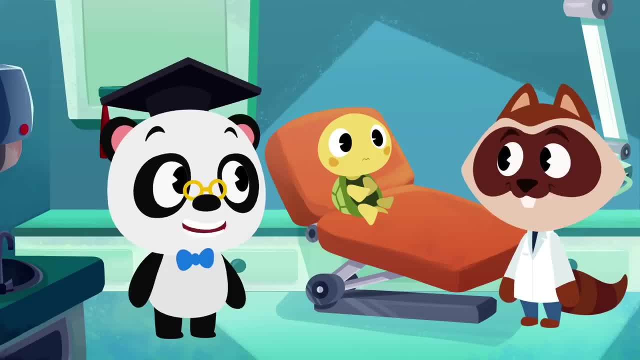 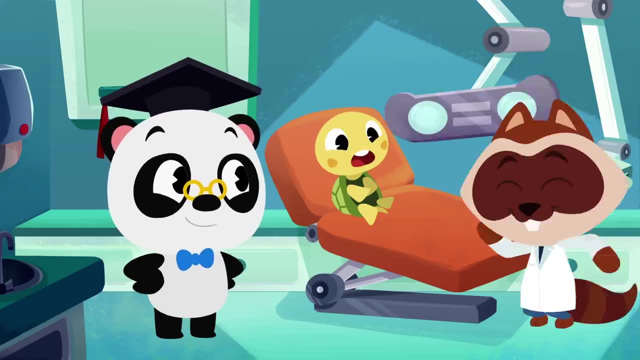 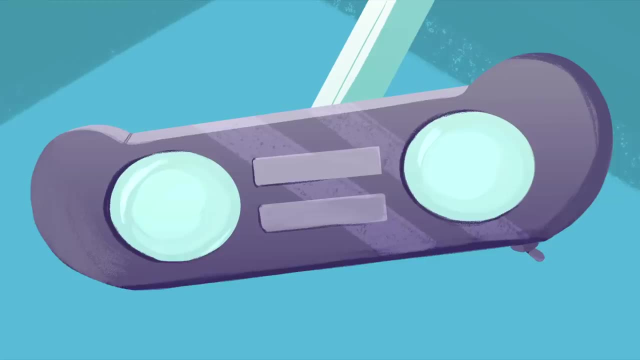 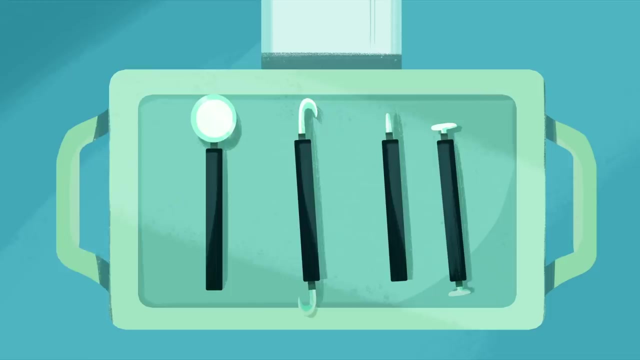 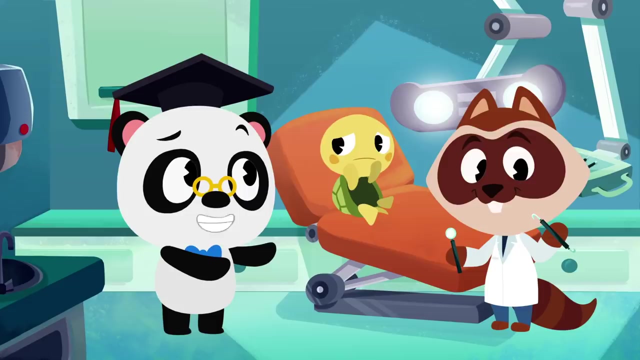 Richie, here is going to have a look at your teeth. You need to open your mouth as wide as you can, Toto, it's only a light. See, You're not hurt, are you? Let's go? Hmm, That's called a dental probe and a mirror. 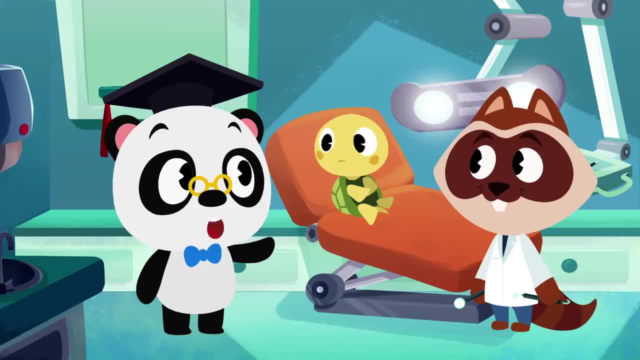 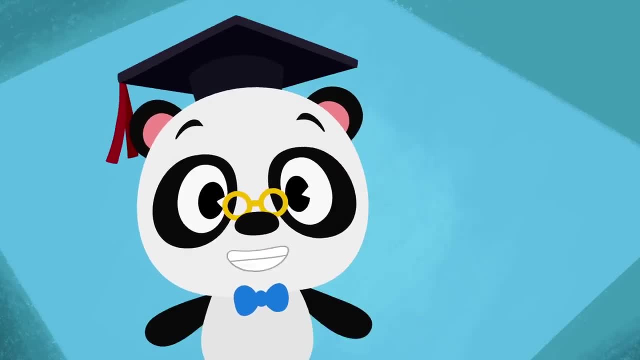 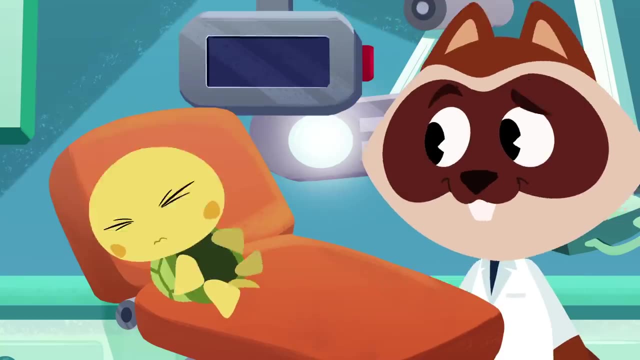 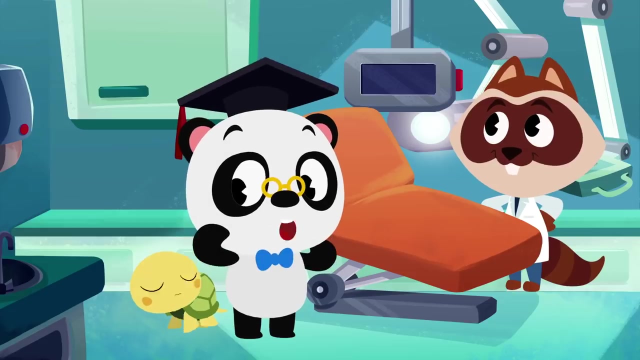 They help, Richie, see the hard-to-reach areas in your mouth. They don't hurt. Look, I'll show you. See, All good, All good. That's only an x-ray machine, Toto. It takes really awesome pictures of the inside of your mouth. 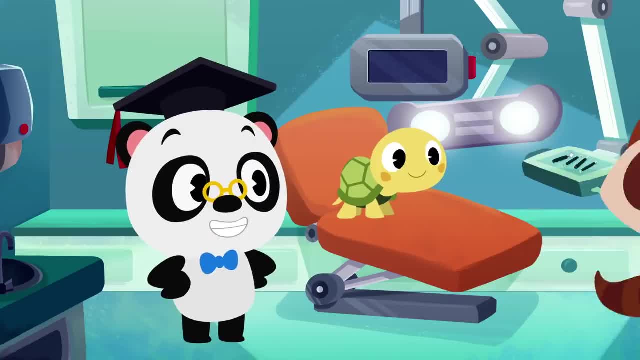 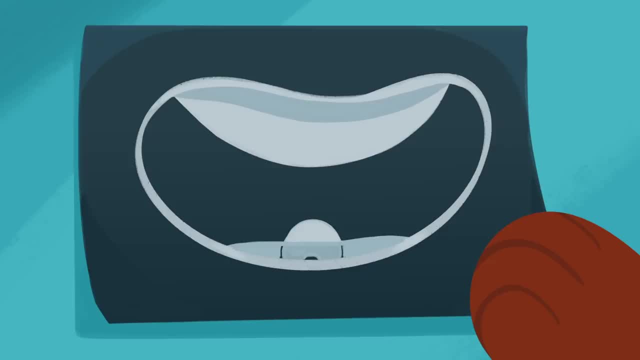 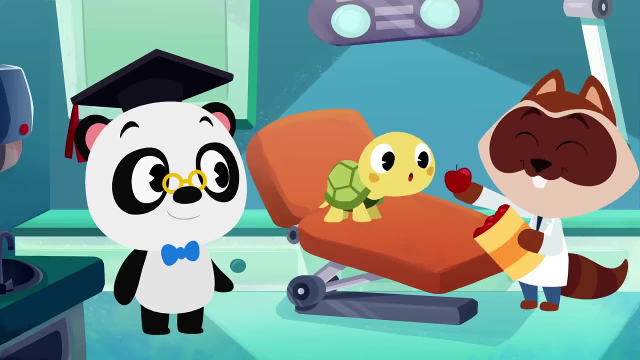 There All done. Oh, I see You have a new tooth growing, Toto. That's why it was hurting Candy. Those are apples, Toto, The best kind of candy you can eat- Yummy Apples. 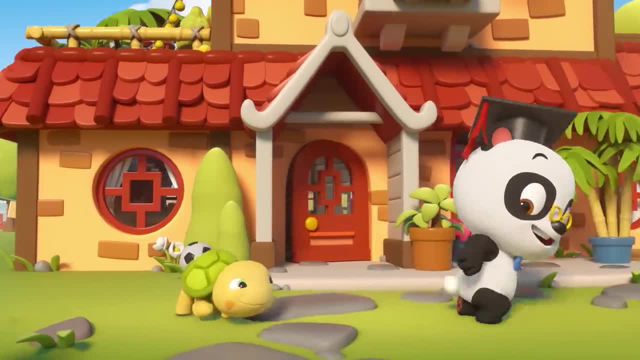 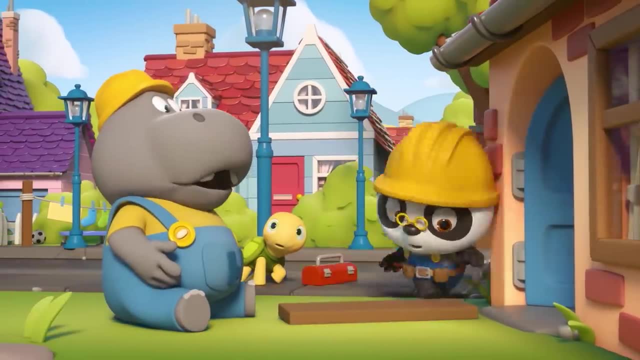 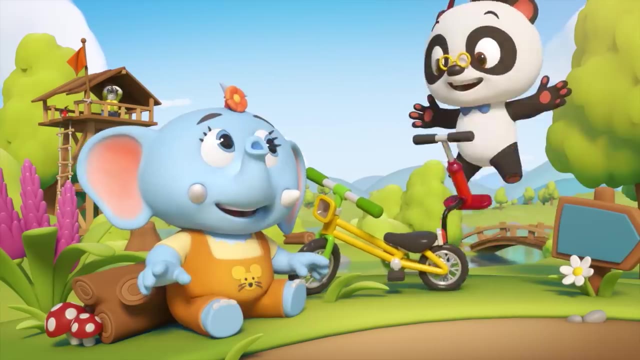 Dr Panda. Hello, Dr Panda, please tell us what will you be doing today. Dr Panda, let's go. Dr Panda, fantastic. come bring your friends and let's play Fighting fires, fixing tires. he always saves the day. 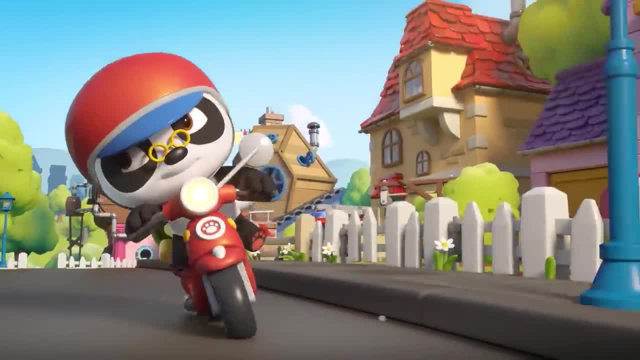 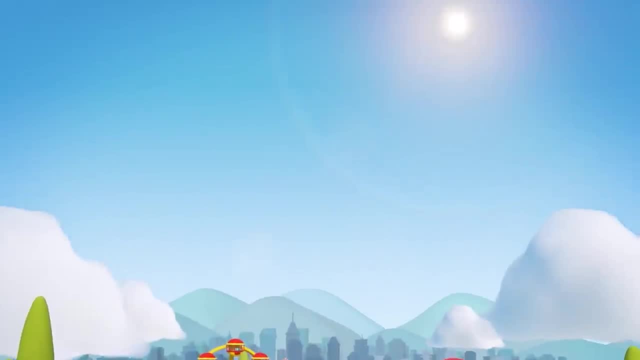 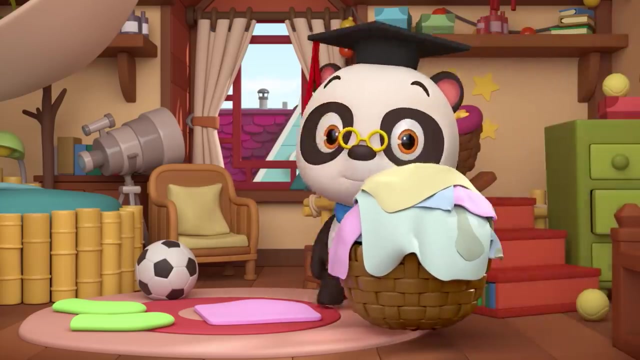 I'll be closer. say no worries, Dr Panda's on his way. Dr Panda, Dr Panda, come on, let's go and have some fun today. Hi, Dr Panda, What are you going to do today? 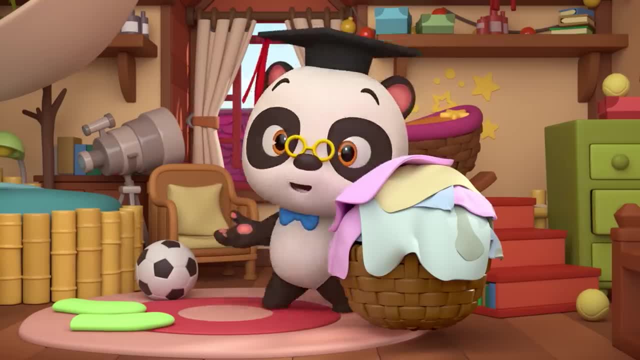 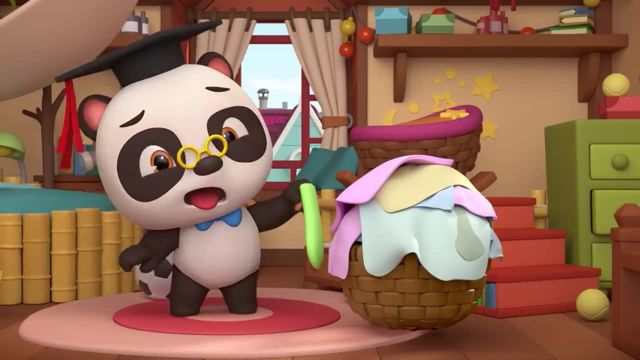 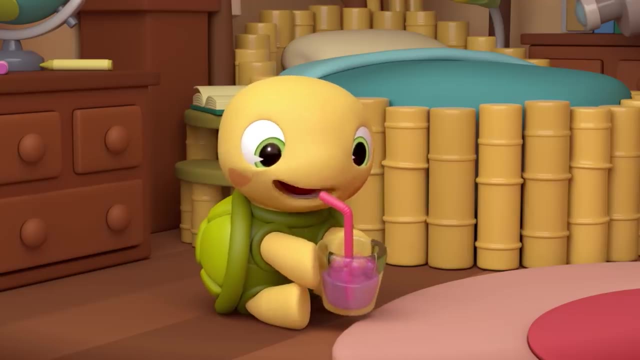 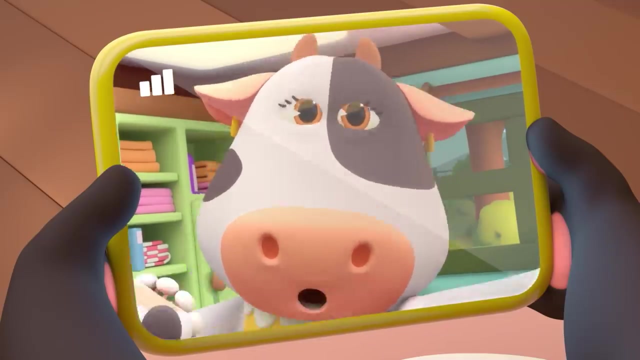 Today I'm going to help Moo with a big pile of laundry. Will you be washing stinky things? Maybe That's a funny noise, Toto Bubbles. Oh hi Moo. Dr Panda, please come now. 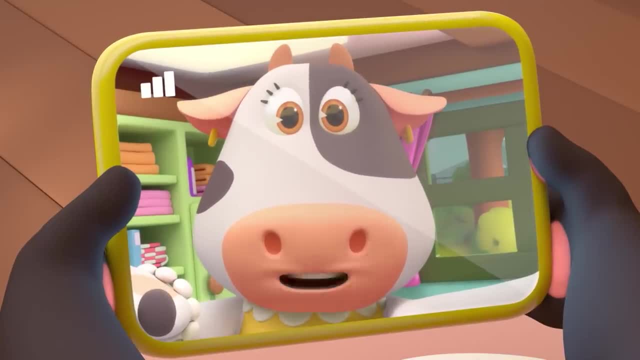 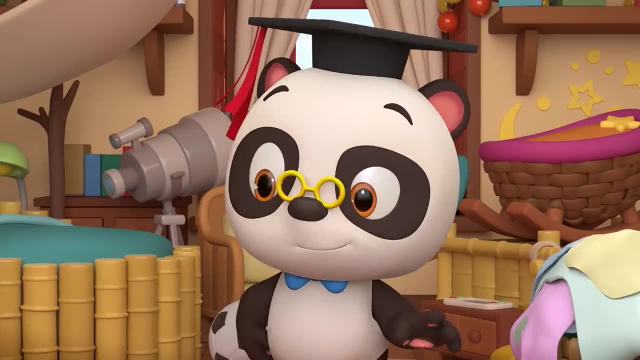 Dr Panda, please come now. Toto and Ziggy's washing machine is broken, so we have to do their laundry too. Oh, there is so much to do. No worries, we're on our way. Are you coming, Toto? 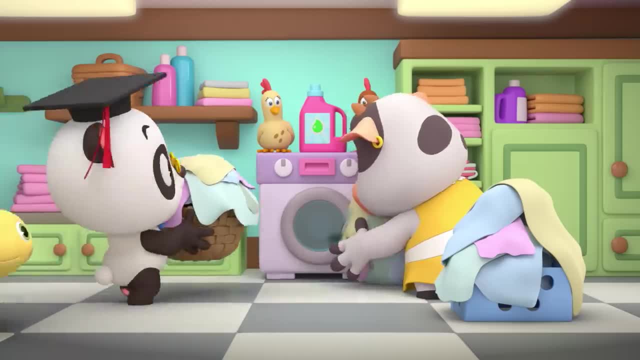 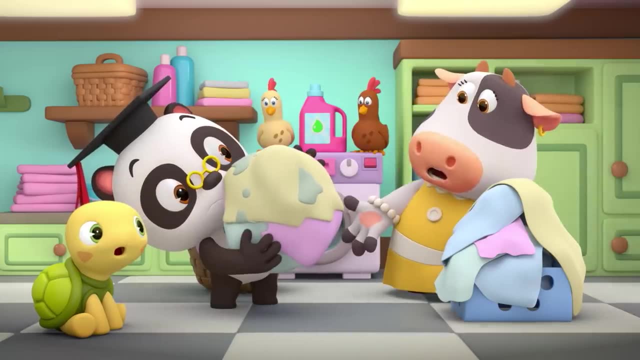 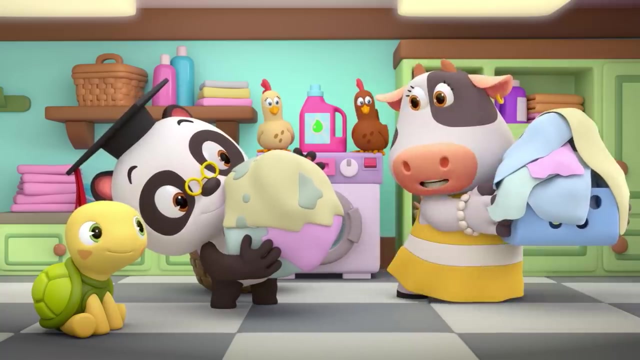 Hi Moo, we're ready to get to work. Oh, thank goodness you're here. I've never seen so many dirty clothes in all my life. No worries, we'll soon have it done. Good, I'll hang this laundry on the line. 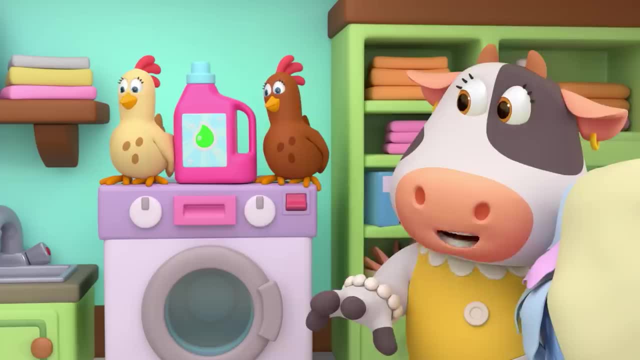 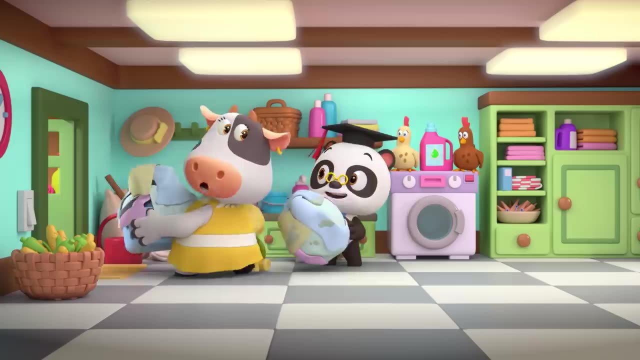 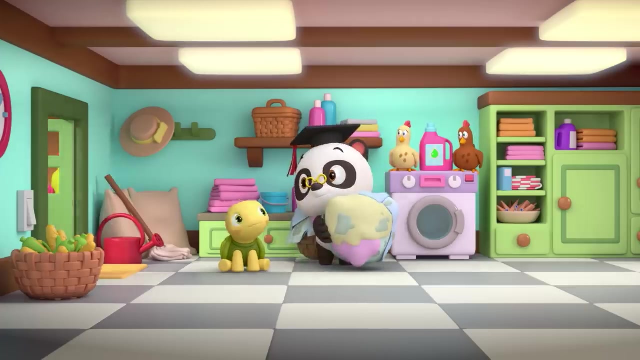 while you put the next load into the washing machine. Great, This is the laundry soap. It makes everything clean and smell nice, but it's very powerful stuff. Only put in one capful per load, Remember, don't put in too much. 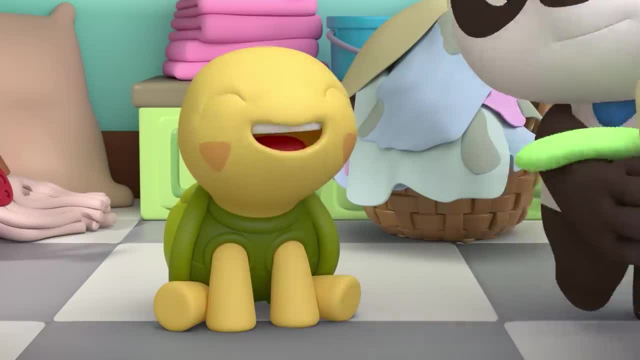 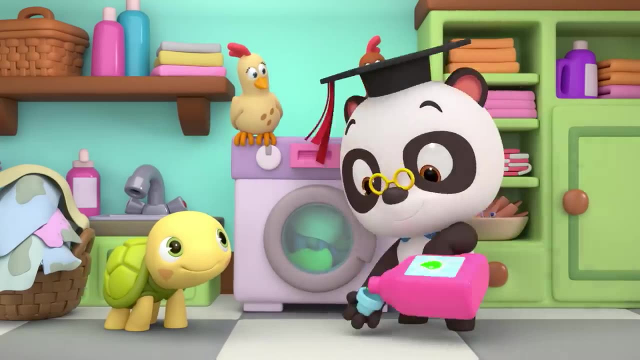 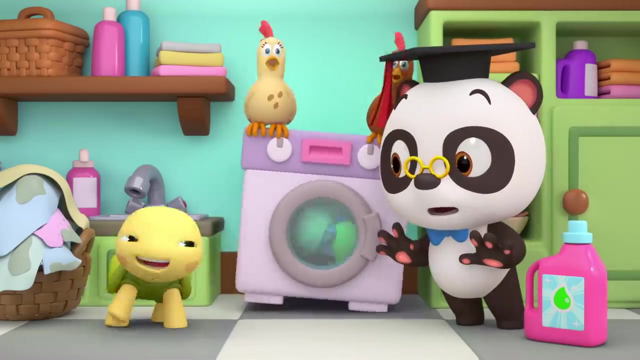 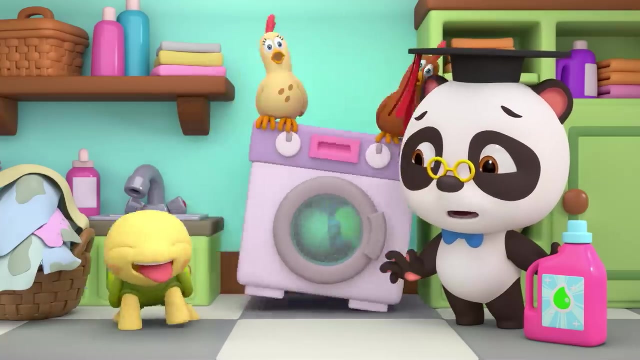 I won't. Let's get this machine going, Toto, Hee-hee, Uh-oh, I don't think it's supposed to do that And it's definitely not supposed to do that. I'd better call Hoopa. 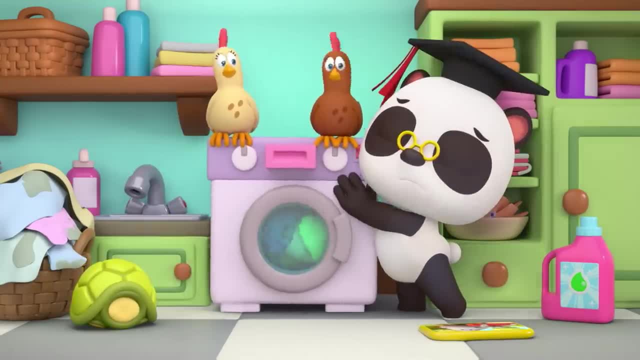 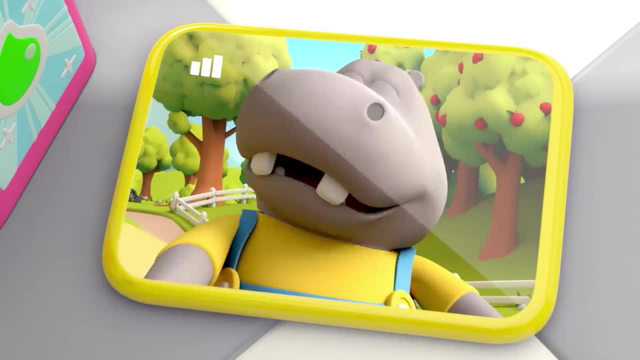 Hoopa, I think Moo's washing machine is broken. Hi, Dr Panda, I'll come round to take a look. I'm right next door. I've just fixed June's fridge, so I've got my toolbox right here. Awesome. 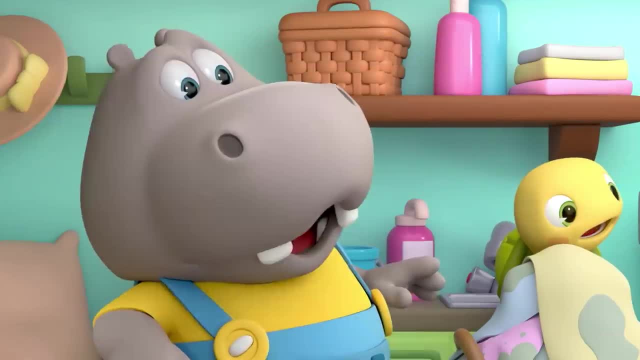 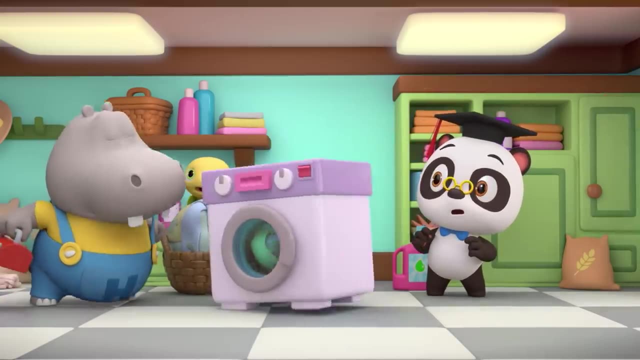 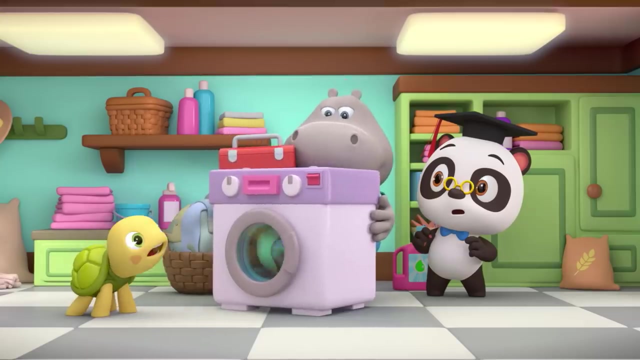 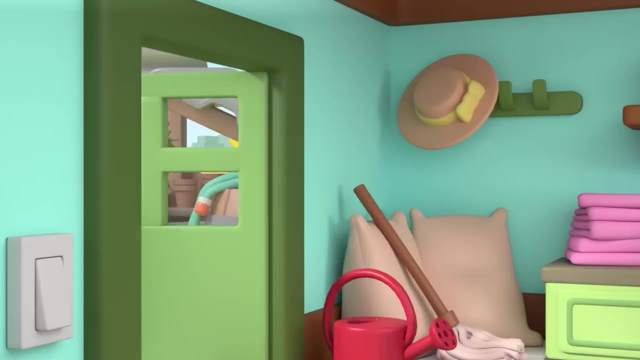 Thanks, Hoopa, Whoa boy. Oh, no Easy fix, Dr Panda. All it needs is something heavy on top to stop it from moving. See, Oh, would that sack be heavy enough? I think so, Dr Panda. help me get the dry laundry off the line, please. 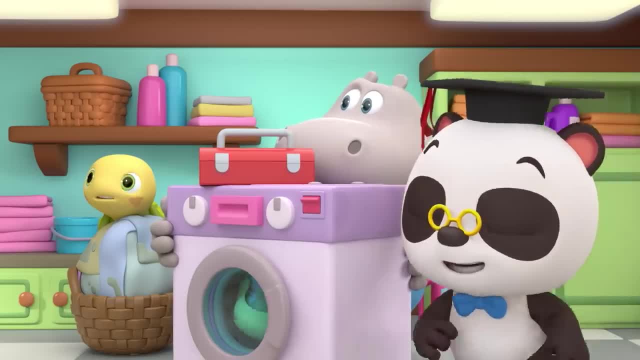 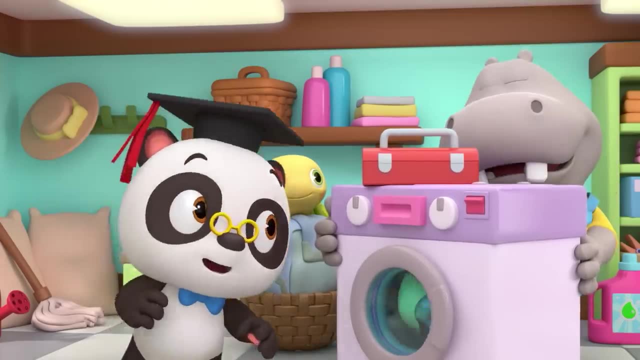 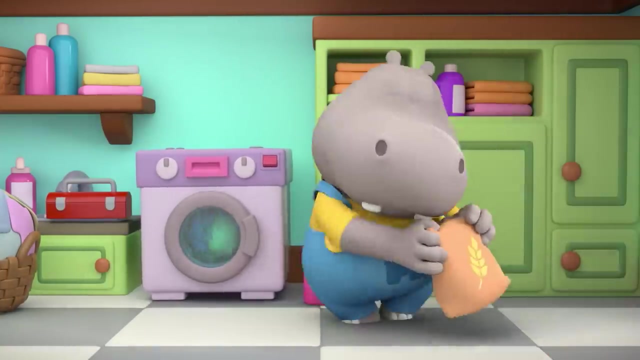 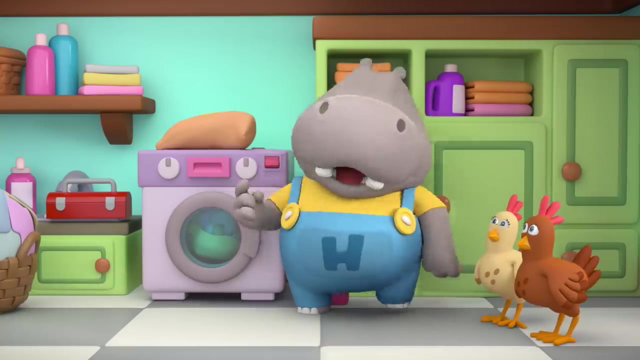 So we can hang up the new load. Sure Hoopa, can you put that sack on top of the washing machine please, Dr Panda, Leave it to me. This load has just finished. I'll put the next load in for Dr Panda. 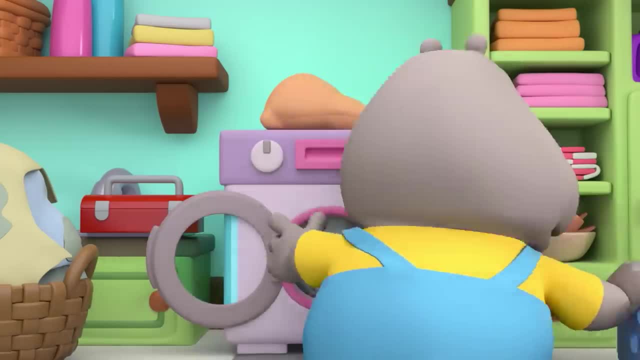 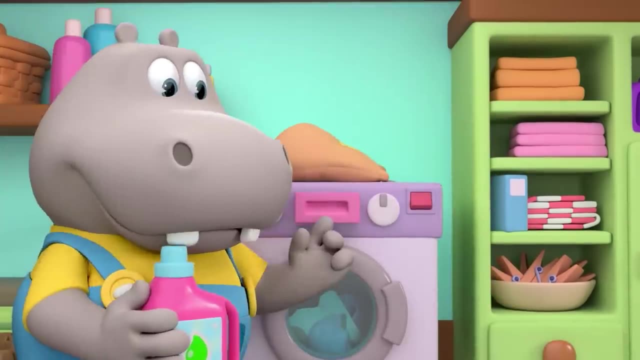 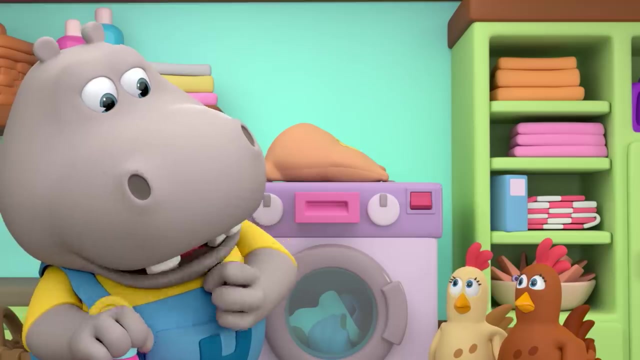 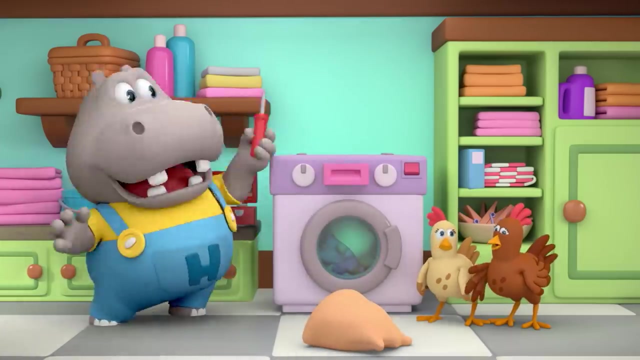 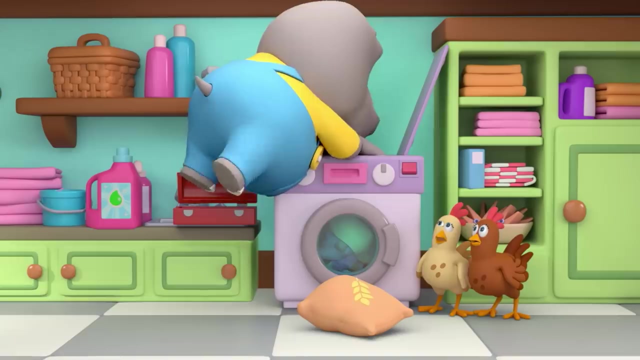 That'll help. Oh, put that in there. Lots of this in here. I reckon I can make the machine go faster. That'd help speed things up There. That'll do it. Hmm, Let's not forget to add this. 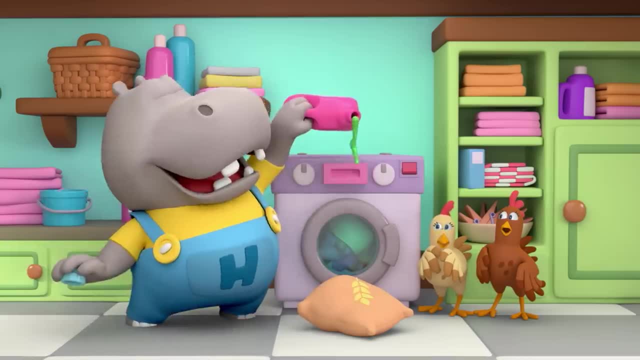 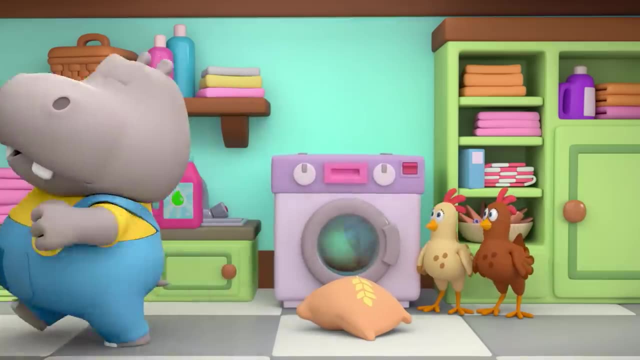 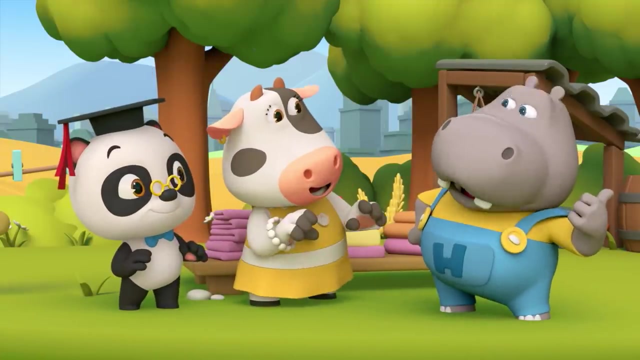 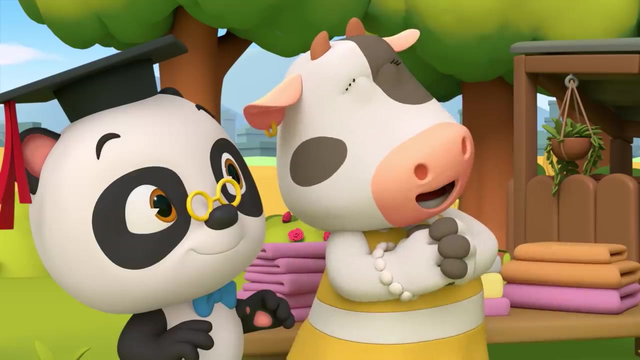 A little bit more, just to be sure. Whoop All done. I gave the washing machine a bit of a boost too, So it'll go faster now. You'll be finished in no time. Oh, that's great. Thanks, Hoopa. 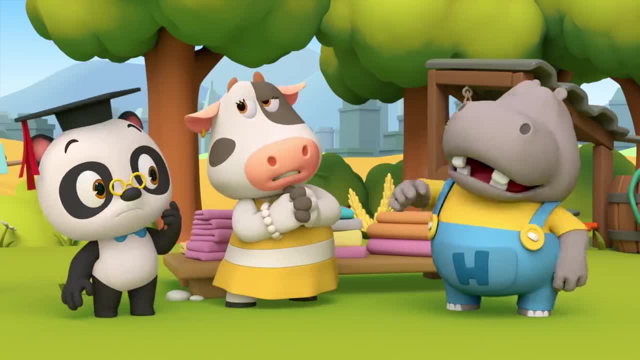 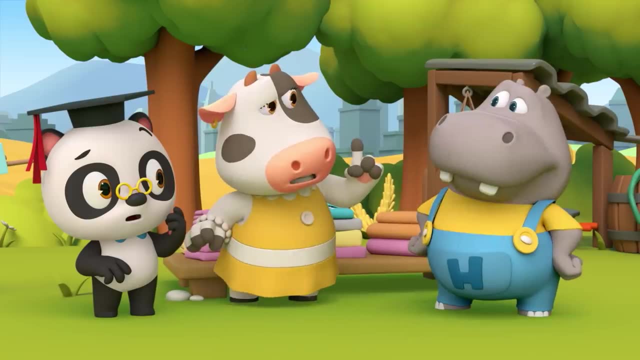 Yeah, Thanks, Hoopa. Ah, What's that? I don't know. It sounds like a machine of some kind. It sounds like my washing machine. Uh, Hoopa, Did you remember to put that sack back on top? Uh, no. 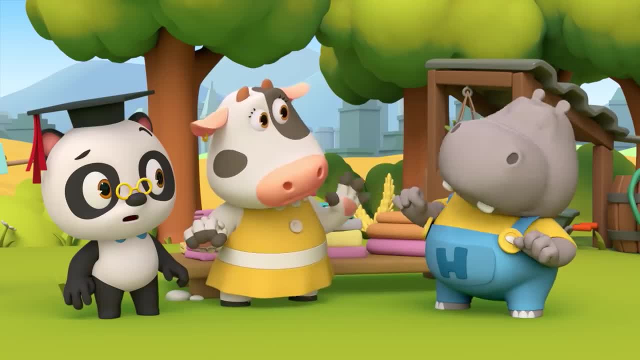 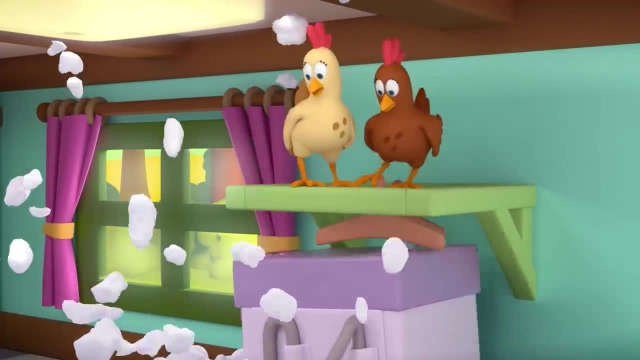 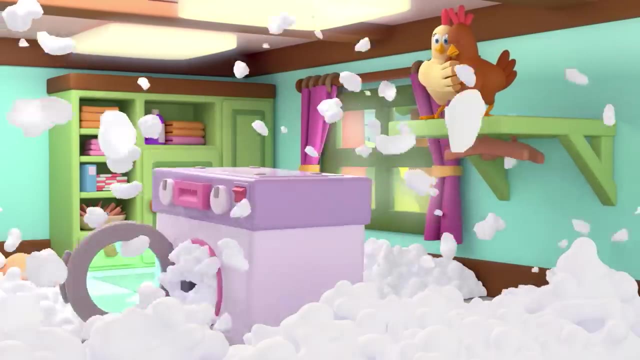 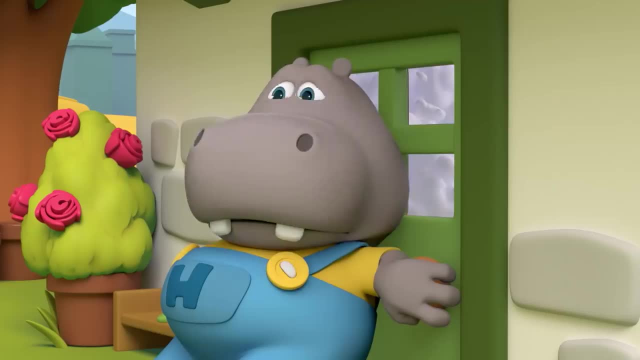 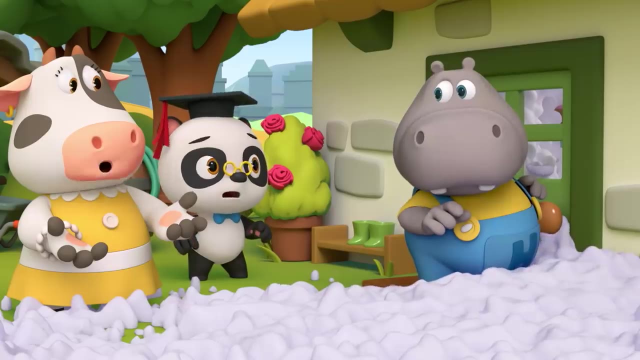 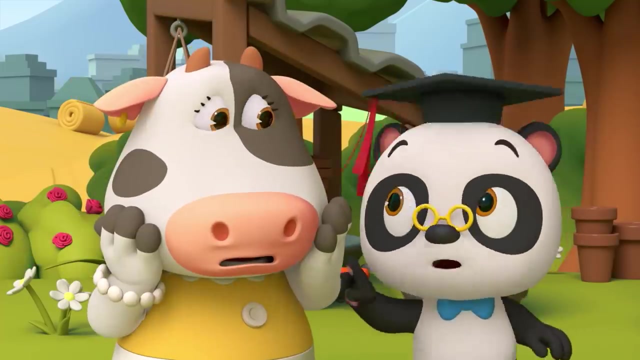 I don't know. It's gone mad. You have to turn it off before it wrecks the place. How much laundry soap did you put in Hoopa? Uh enough, This is a disaster of something. would you better? otherwise my whole farm is gonna be covered in bubbles. 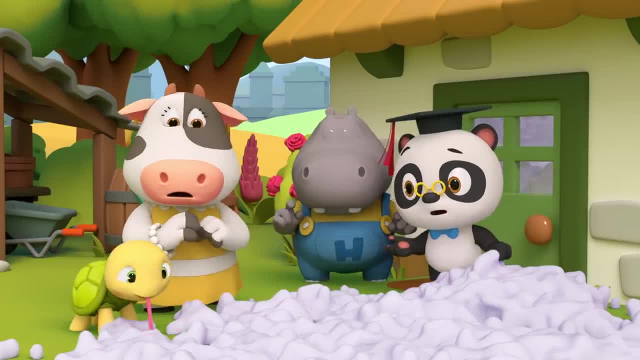 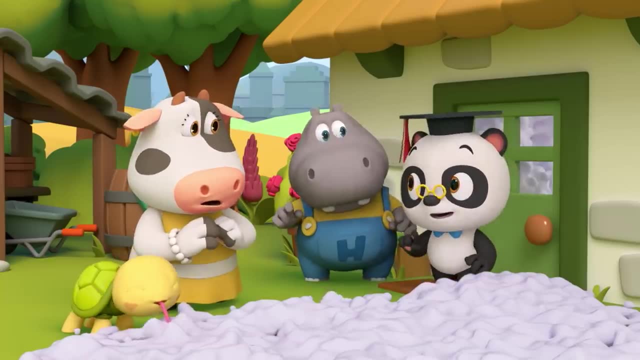 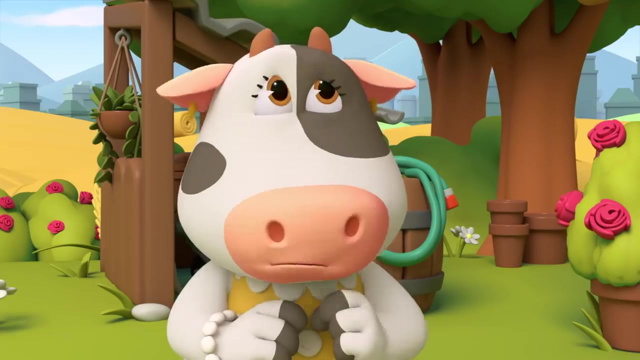 i can't even see where the machine is. oh, that's it. toto, i've got an idea. you have, you have. yep. thanks to toto moo, have you got those swimming goggles from your vacation? um, yes, hoopa, can you hand me those hoses behind you? yep.